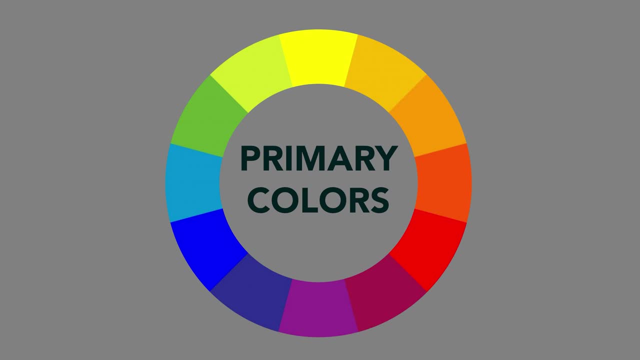 about primary colors, of which there are three. We have red, that is a primary color, yellow, that is a primary color, and blue, that is also a primary color. It's these three primary colors, then, that we use to combine together and make the secondary colors. We have green, we have orange and we have 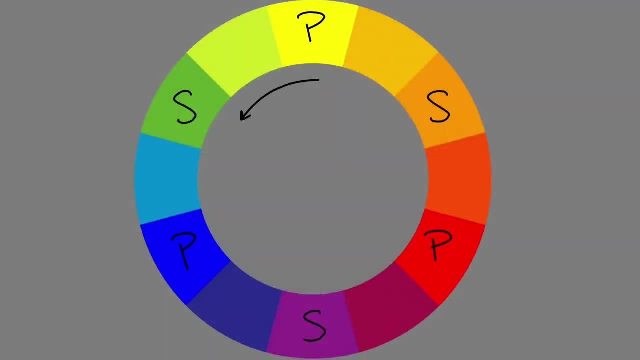 violet. If we take our primary colors and mix them with another primary color, we're going to wind up at a place where we have one of these secondary colors. So yellow and blue together makes green. yellow and red together of course make orange and red mixed together with blue is going to give us. 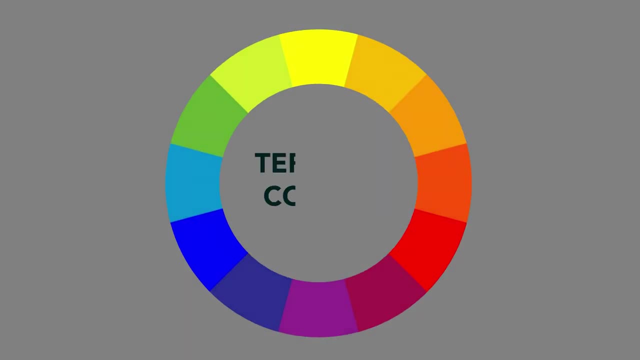 violet. So far, super simple. right Now, a tertiary color is essentially two additional steps down the line from a primary color and we get them by mixing together a secondary and a primary. So yellow mixed together with green is going to give us our first primary color, and yellow mixed together with blue is going to give us our secondary color. 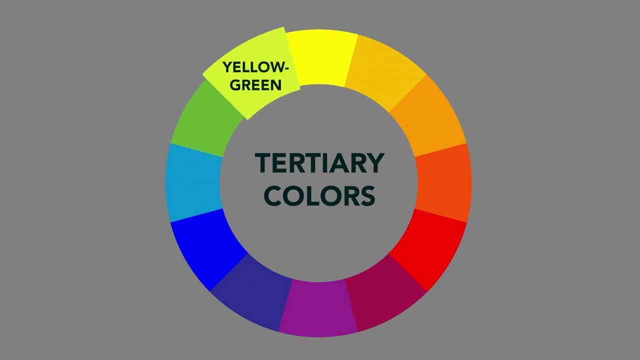 So we have our first tertiary color, and that is yellow green. our second tertiary color is yellow orange. our third tertiary color is red orange. after that we have red violet, we have blue violet and we have blue green. So, to review, we have three primary colors. we also have three secondary colors. 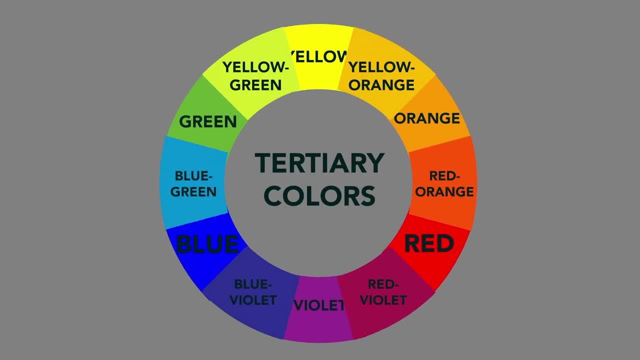 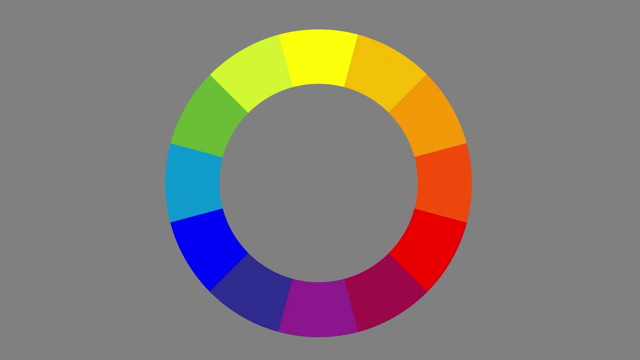 and we have six tertiary colors. This is color wheel vocabulary at its most basic. The next thing we're going to talk about in this most basic color wheel that we have here is something that I think is probably one of the most important topics that you'll need to assimilate moving forward, and that 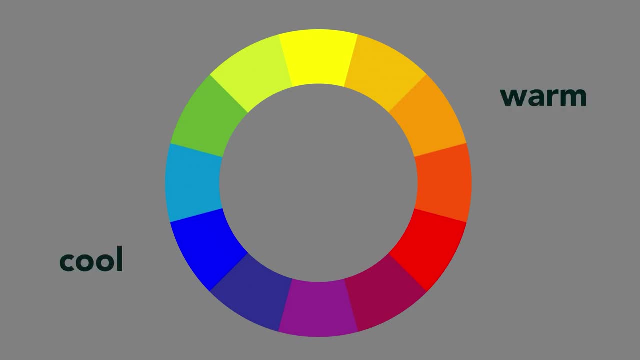 is understanding the basic divide in between warm and cool colors. Now, this is a technical division. we're not talking here about colors that feel warm or conjure up some warm emotion. we're talking about proximity on the color wheel to blue or to orange. What I'm going to do is split the color. 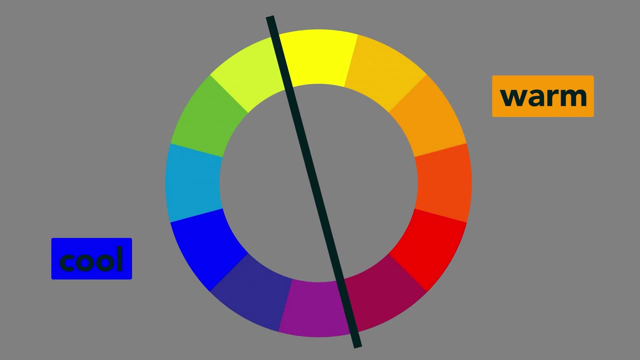 wheel down this axis. On one side of this, we have warm colors and on the other side cool. There's probably a lot of different ways to do this, but I'm going to show you how to do it, So let's get started. 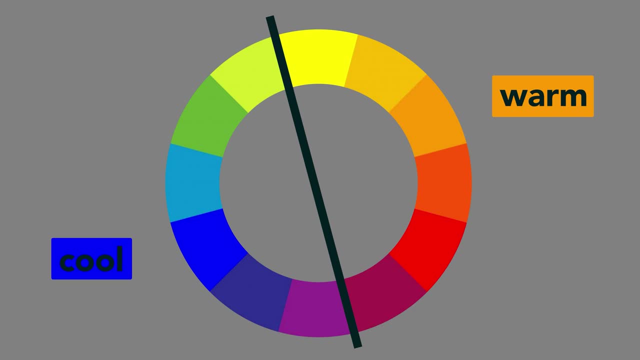 There are a few ways that we can explain the warm cool concept, but let's just say that colors that contain some noticeable quantity of blue are going to be considered cool, whereas those not containing that noticeable quantity of blue are going to be warm colors. Now why is the warm cool distinction? 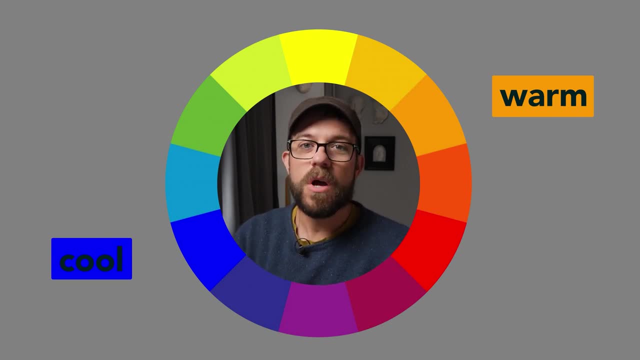 so important. It defines a lot of the different effects that you're going to be shooting for when you're making your oil paintings. Colors appear most lively to our eye when they're juxtaposed against their opposite. Some of the compositions that I'm going to show you later. 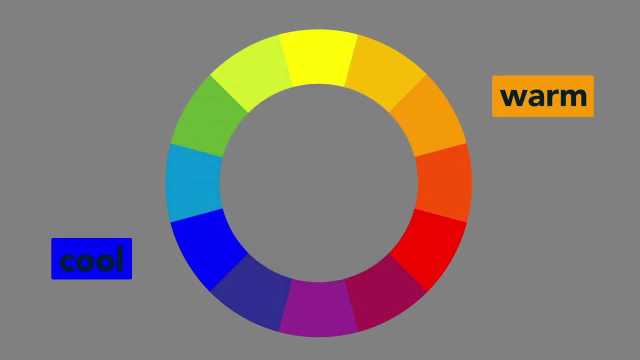 really bear this out. Oftentimes you'll find a large quantity of analogous warm colors juxtaposed against a small amount of something cool. that creates a kind of accent and activates the warm side of the temperature scale. Let's talk analogous colors, If we have. 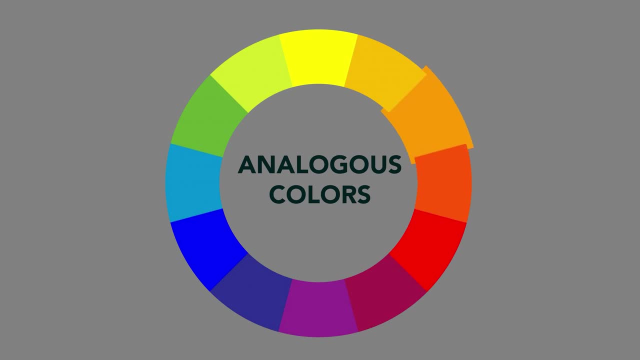 one color that we start out with, the colors immediately flanking it on the color wheel are analogous to that color. So in this case, yellow, orange, red, orange and orange are analogous colors And all of the other colors on the color wheel follow suit with that same idea. 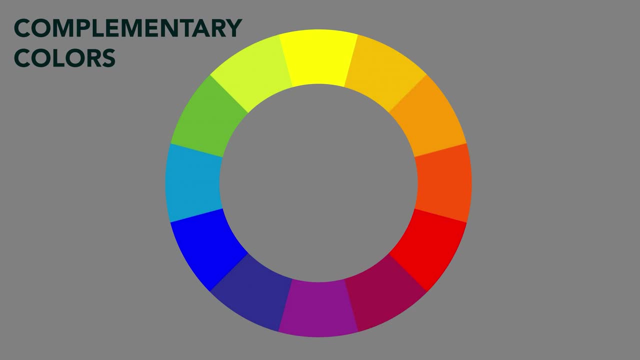 Now let's talk complementary colors. A complementary color is the color that we find across from another on the color wheel. It's interesting to note that the three primary colors do not have complements among themselves. They are essentially a triad, But once we include secondaries and tertiaries, we have opportunities to have. 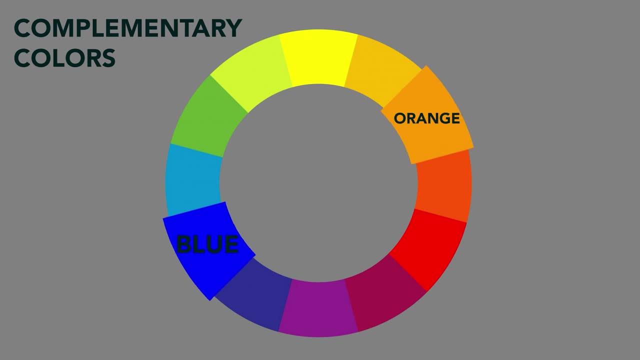 complementary colors. The complement to blue, then, is going to be orange, yellow is going to be violet, red is going to be green, blue violet is going to be yellow orange, red violet is going to be yellow green and blue green is going to be red orange. The reason it's important to 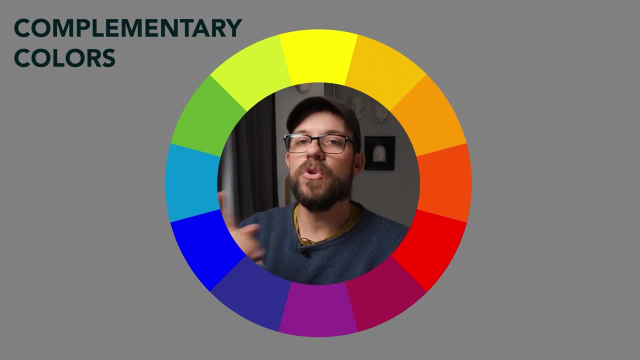 know the mechanics of complementary colors is because one color will actually neutralize the other in terms of saturation. So if we have a very highly saturated yellow and we want to neutralize it, we would reach for whatever we had on the palette that could equate to a violet, A lot of. 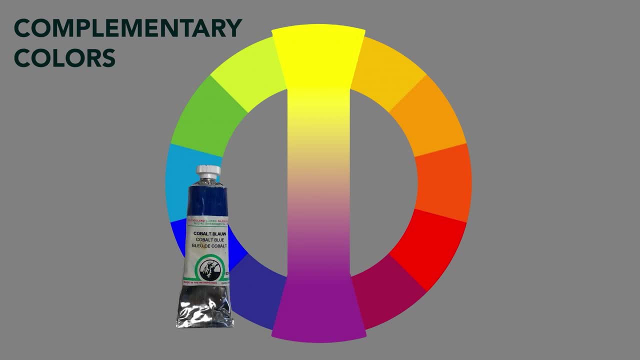 times. in practical terms, that's going to be a mixture of something like a cobalt blue and a vermilion. Mix those two together, you essentially get the most violet color you can, which will act as a complement to yellow and will thus decrease or neutralize the. 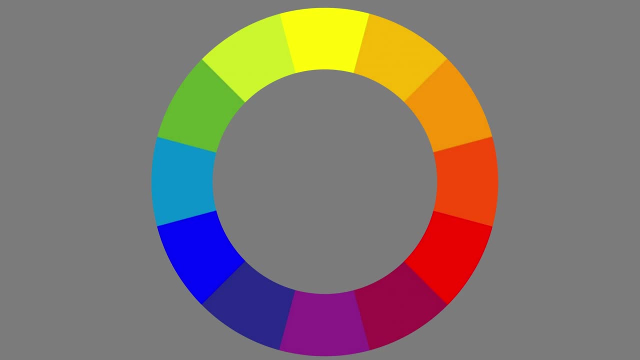 of that yellow. The next word we're going to define I think gets misused a lot. I'm going to talk about the word hue. A lot of times people will use the word hue to describe a color. They'll say that orange is a hue, red orange is a hue, red is a hue, And while that's not entirely incorrect, 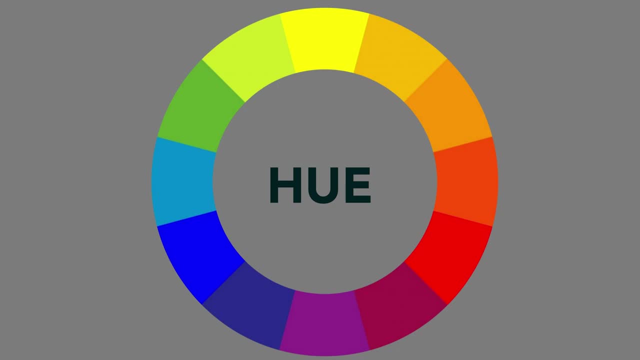 it's also not quite specifically what hue means. The word hue describes which of the 12 wavelengths of color is the dominant wavelength of a color. It becomes important because, eventually, a lot of the colors that we see aren't presented to us in such a way. 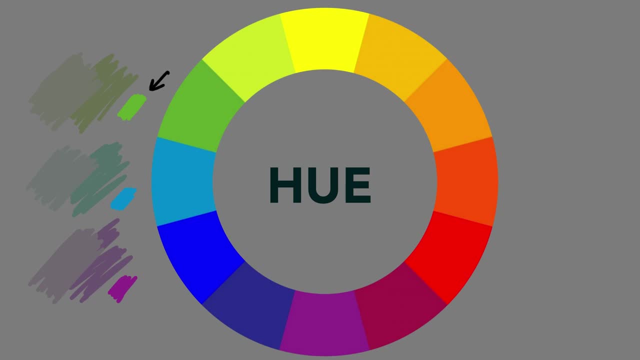 that they are at their purest expression. A lot of times a green in a painting or in nature will be expressed in a very low saturation, which almost makes it look like a gray. But here we can still say this is a green because the dominant color in that mixture, the one that really stands out. 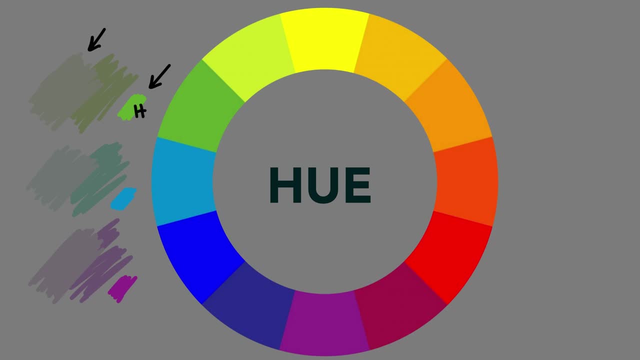 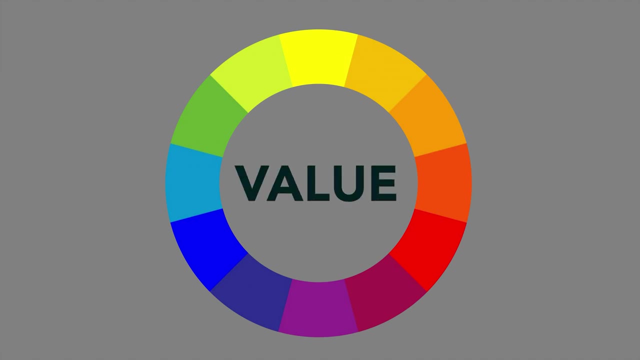 is green, So in this case, the hue is green. Also, in this case, the hue is green. The next thing you need to know is value. What do we mean when we say the word value? What we're talking about is on a gray scale. what is the lightness or darkness? 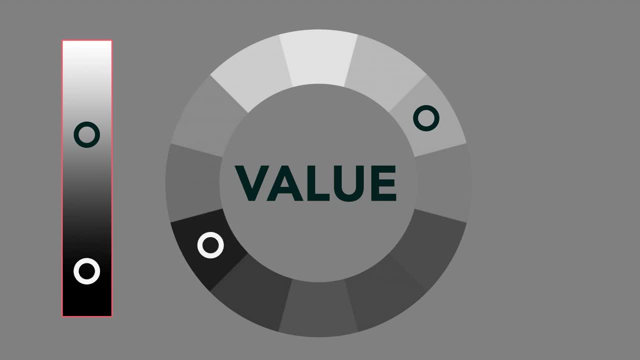 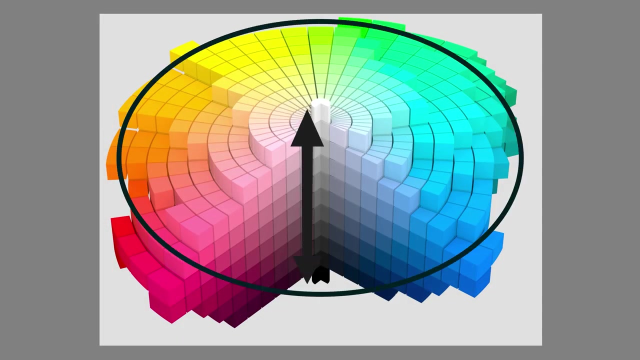 particular color. Each of the colors, then, is assigned a specific value. This becomes particularly important for an oil painter, when you're trying to balance hue, value and chroma without making your mixture too dark or too light. Now we've talked about value and we've talked about hue. Now I want to 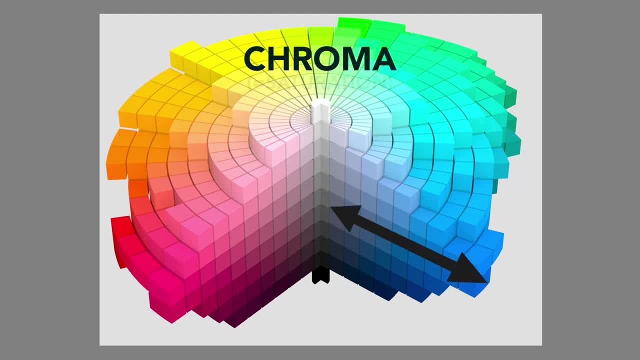 talk to you about chroma. You could say chroma is almost synonymous with saturation, And what we're talking about is how pure the particular expression of a color is. When we talked before about hue, we said: what is the dominant color inside the 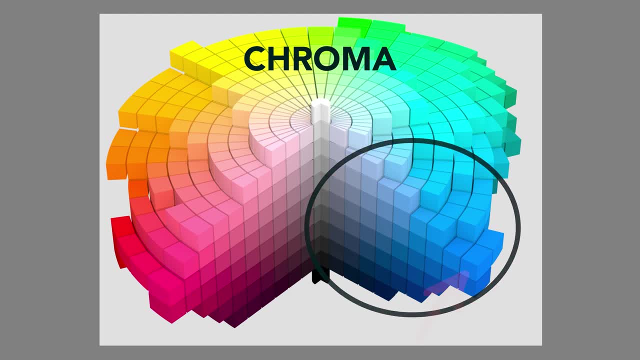 mixture. In this thread we clearly have blue Down. here we have a highly chromatic blue. Here we have a very desaturated or low chroma blue. Nonetheless, the hue is blue. Here we have a high chroma blue. Here a low chroma blue. Eventually, in my 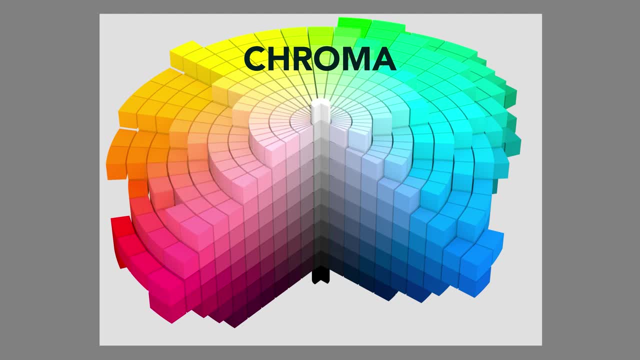 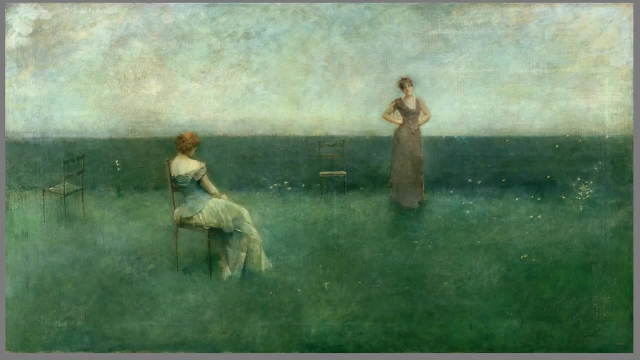 practical color lesson. you're going to hear me talking about high chroma mixtures, or high chroma colors and low chroma colors. This, then, is what I'm talking about. in that context. We have a fantastic painting by Thomas Wilmer doing Here we. 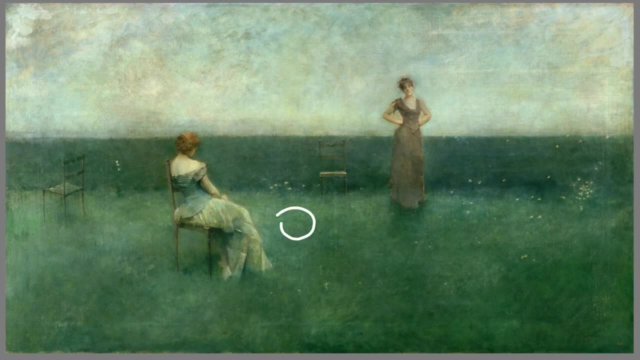 have a highly analogous color scheme. We have lots of greens, we have lots of blues, we have lots of full greens, we have lots of blue greens And, of course, we have a typical but desaturated blue in the sky. All these colors then have a relatively 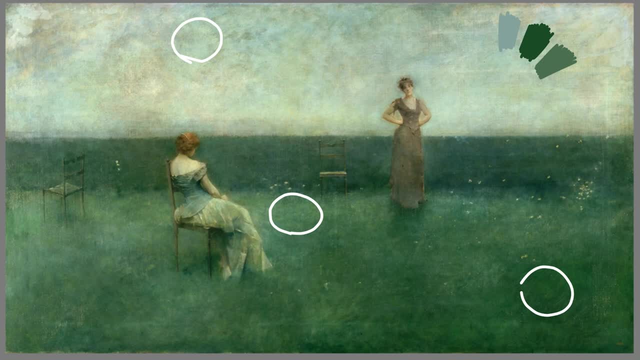 tight relationship in a color space, But are they all alone? Is it almost a monochromatic composition? Absolutely not. Doing draws your attention to one of the central characters. by doing what? By choosing a complementary color for the hair of his model. 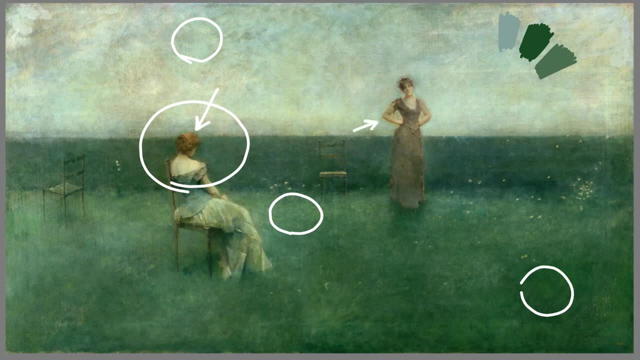 In addition, we find small notes of orange, also in the other model, inside of an overwhelmingly cool context. What we end up with in the end is something that is tantamount to a complementary color scheme in this painting: An overwhelming proportion of cool balanced by a small and therefore much more. 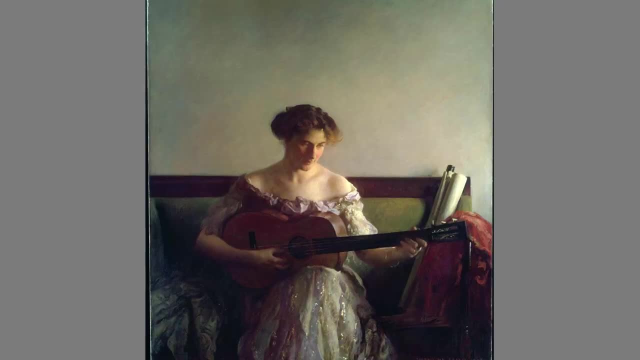 noticeable presence of very warm temperature. Finally, we have this painting by Joseph de Camp. I chose it because he's created a very beautiful harmony of a vast variety of different hues. We can find strong chromatic reds. we can find chromatic greens, we can find 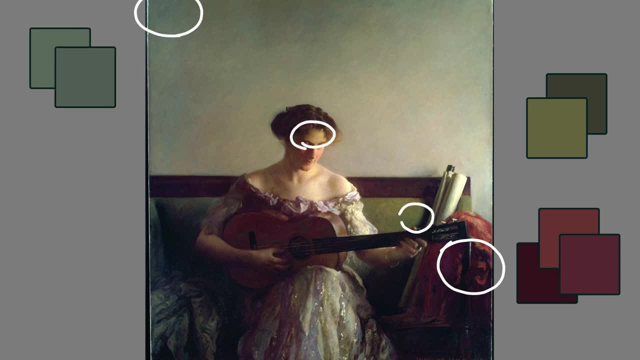 soft but saturated blues, the yellows of some of her flesh tones, And though each color is relatively strong in its ultimate expression, here we find that they all harmonize really, really well. There can be a lot of different reasons for this, But what I want to point to here is a concept that 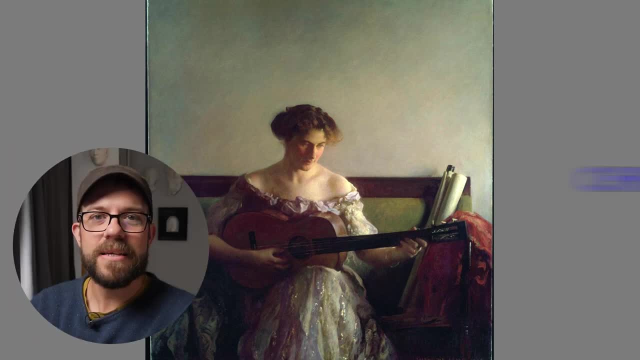 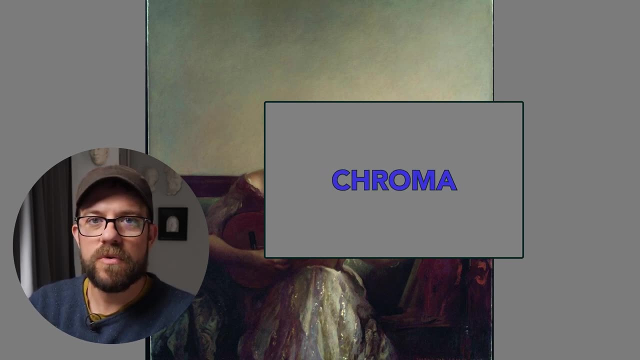 I heard about Vermeer years and years ago. It's about color, intensity and proportion And it said that in a picture they should have an inverse relationship. The more chromatic the color that you use, the smaller amount of space it should occupy and therefore the larger amount of space the color. 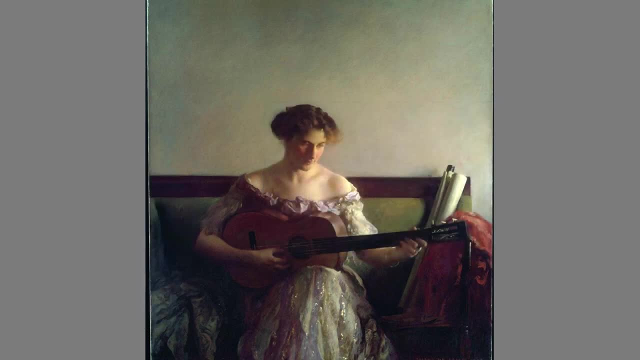 is occupying, the less chroma it should have. So what do we find in this massive background? behind her, We find relatively low chroma hues, And where do we find our highest chroma in the various hues that are represented here? Relatively, 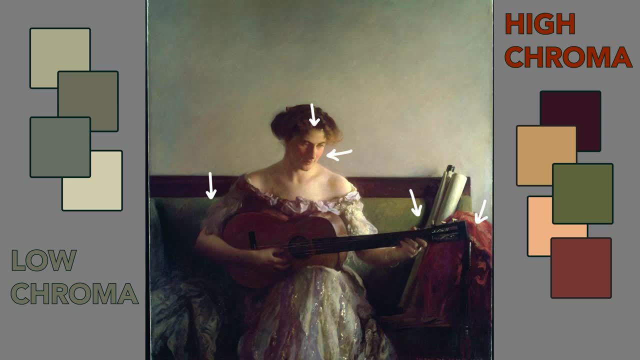 small and discrete areas that he wants to draw particular attention to. I wasn't there, of course, when de Camp designed this painting And I can't say that chromatic proportion was in his mind when he did, But I can say that over the years throughout. 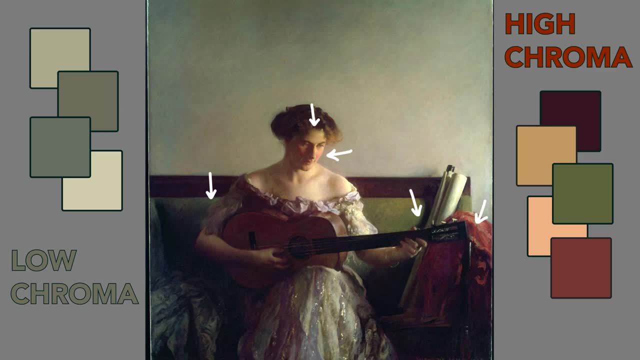 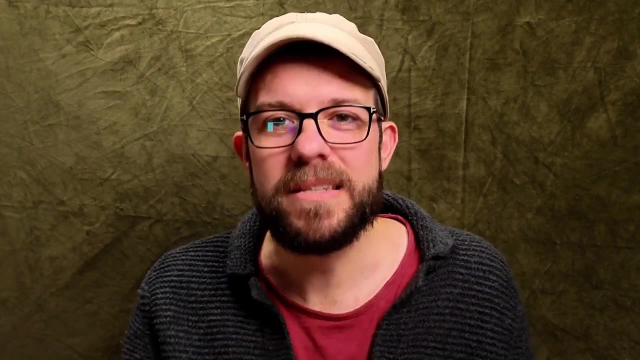 the arts and art history he's drawn to chromatic proportions on color theory fundamentals. If you're interested in learning all of the rest of the stuff that I cover in this lesson, you can follow the link in the description of this video to my 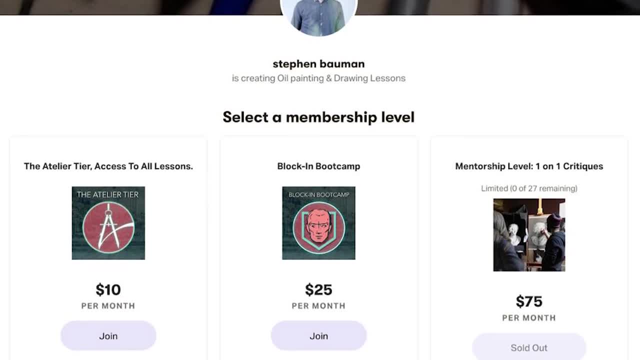 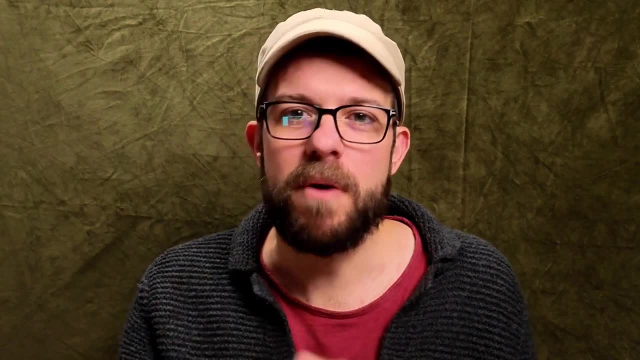 Patreon page, where you will find it at the atelier tier. That being said, at this moment you should feel prepared with the basic vocabulary. you need to figure out how to work as an oil painter in the world of color and use color theory to better. 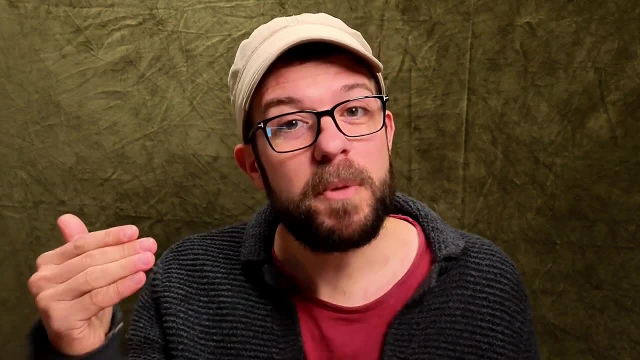 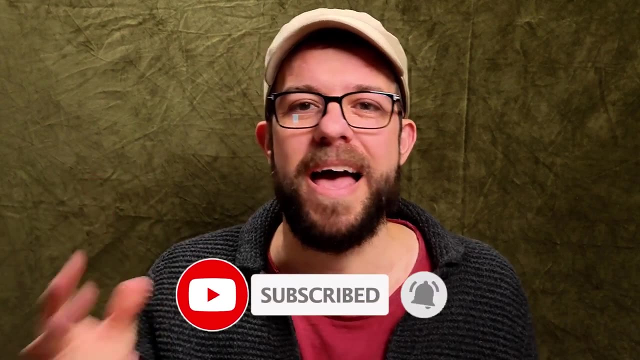 express yourself as an artist. Anyway, I want to thank you so much for watching. I'm Stephen Bauman And if you like the content here on this channel, please remember to like the video and subscribe to the channel and I will see you on. the next one. 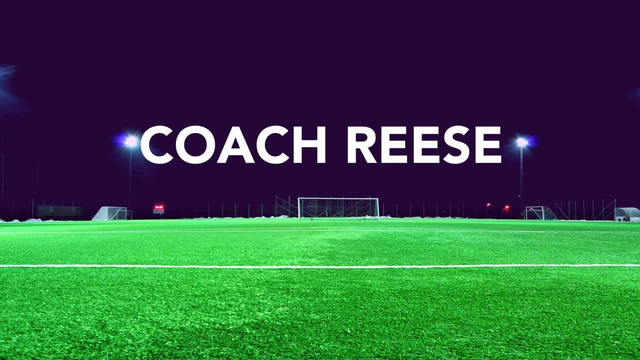 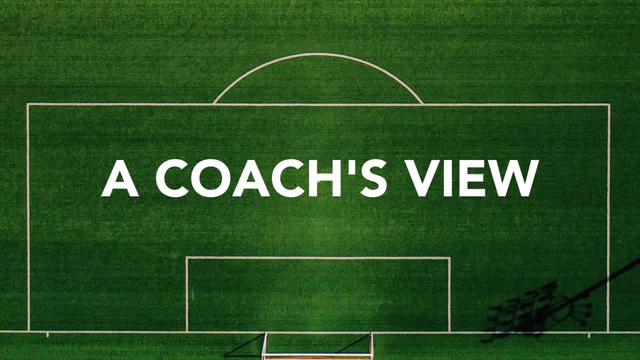 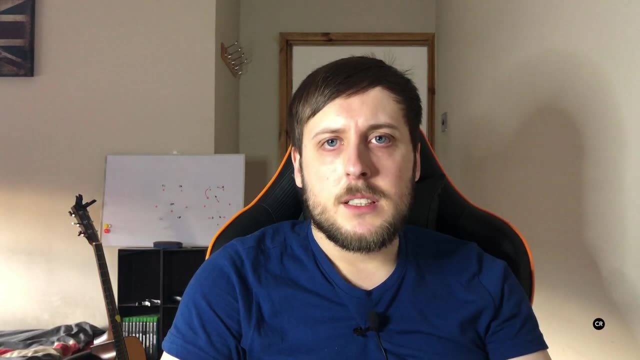 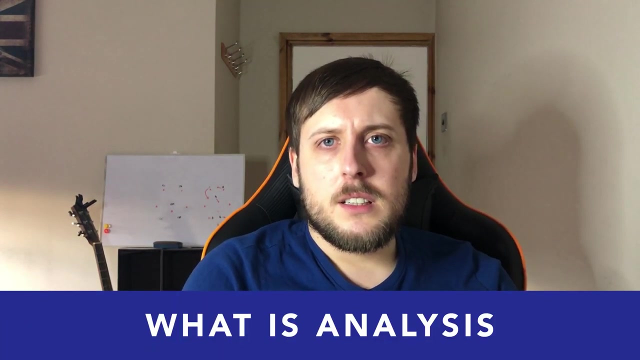 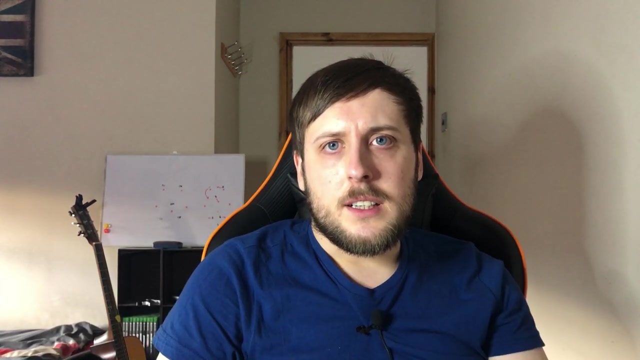 In today's video we're going to talk about how you can analyze football matches, But quickly, before we get started, help a coach out, hit subscribe. So what is analysis? Analysis is essentially watching the game and drawing conclusions from what you're seeing, and that does sound pretty easy, but it can be quite challenging, especially. 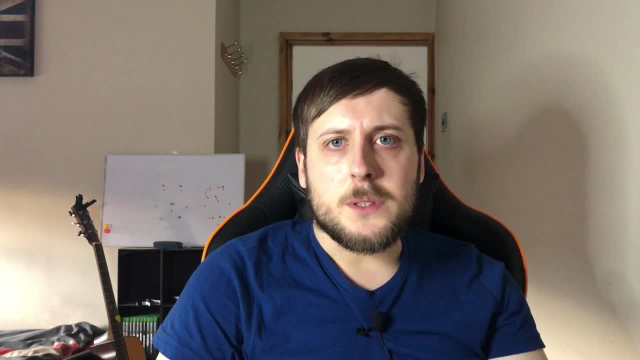 if you're very new to it. So what we're going to do is we're going to break it down into small sections that, once they all come together, you'll have an excellent piece of analysis. So to help us with this, we're going to break it down into three steps and I will leave timestamps. 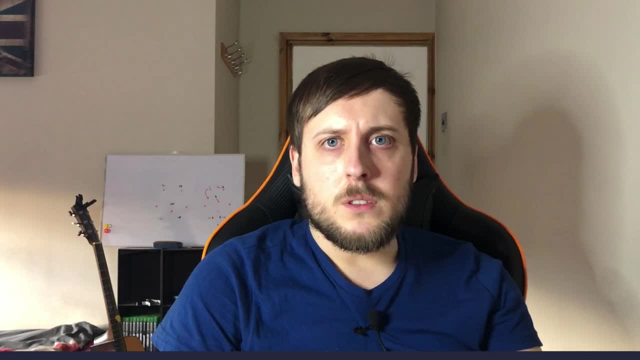 to each step in the description below. So step one is pre-game and it's a part of analysis that's often overlooked because it's not actually the game, but it's incredibly important and it's a little bit cheesy. but fail to prepare, prepare to fail. It's quite fitting for analysis. 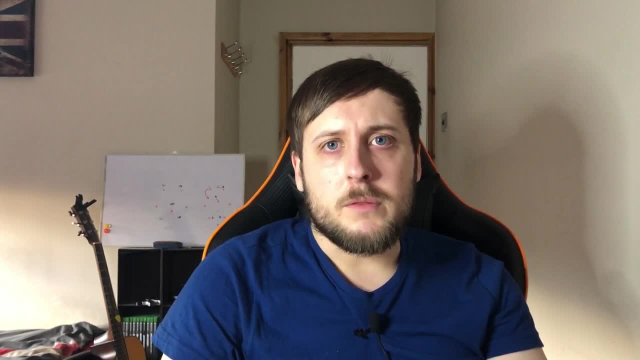 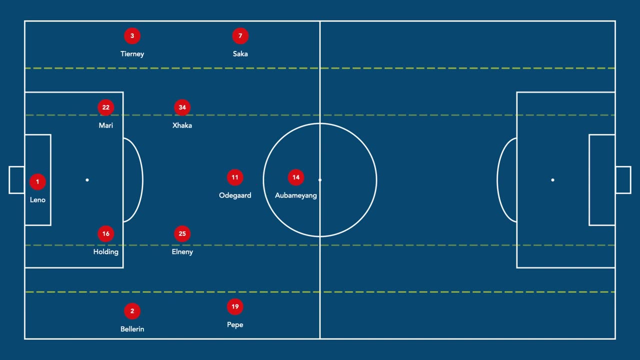 so if you don't do this pre-game, it will affect the analysis of the actual game. The most important piece of information that you need to get pre-game is the formations of teams and kit numbers and player names, if you need them. if it's a team you've not watched before.